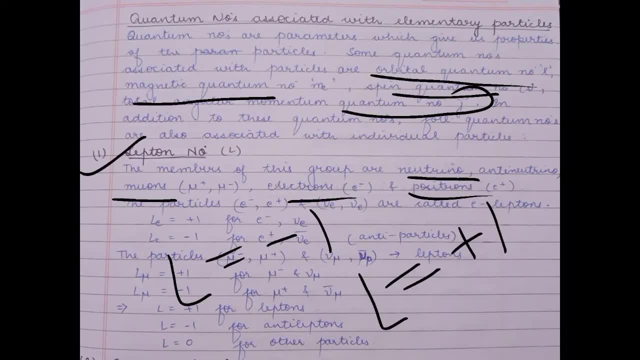 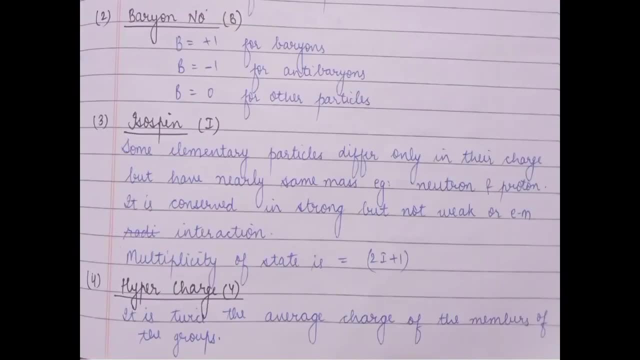 particles which are not the leptons, the lepton number L will be equal to 0.. Now another quantum number is baryon number. As we have lepton number for leptons, similarly we have baryon number for baryons. We know that baryons are nucleons and hyperons For these nucleons. 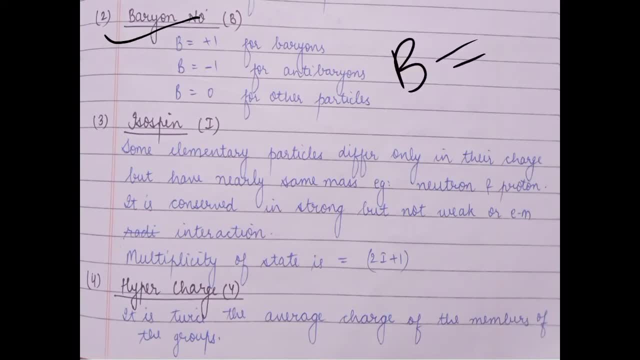 and hyperons, we have B equal to plus 1.. That is, baryon number is equal to plus 1, and for these antibaryons we will have B equal to minus 1, and for these antibaryons we have: 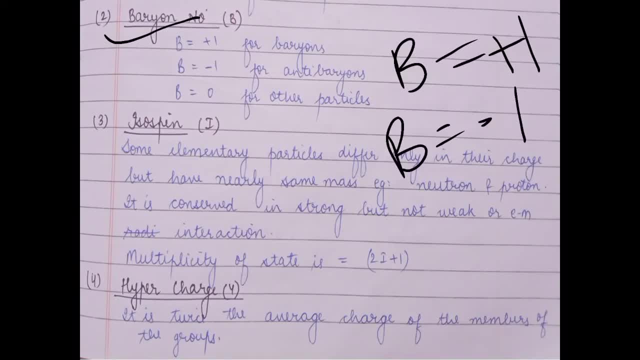 b equal to minus 1, and for all the other particles which are not baryons, for example for leptons, for photons, the b value, that is a baryon number for all other particles except the baryons, will be equal to 0.. Now another quantum number is isospin. Isospin is a quantum number which give. 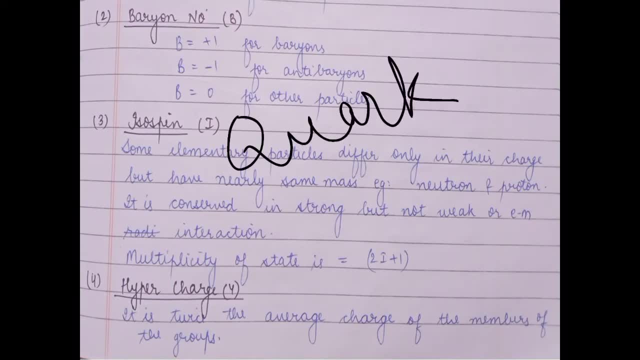 us the quark composition. We will study about the quarks in later videos. We know that some of the particles differ in their charge but have nearly same mass, for example neutrons and proton. We calculate isospin by the formula 2i plus 1.. We will see the isospin numbers in few seconds. 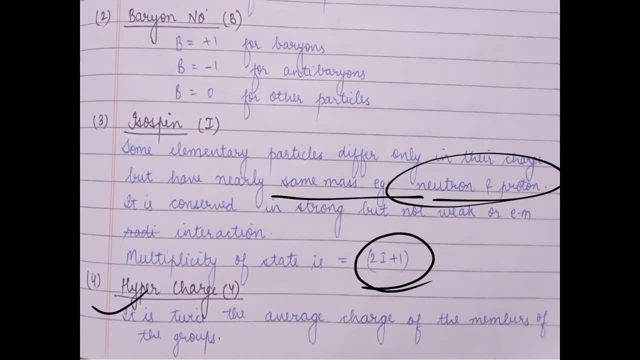 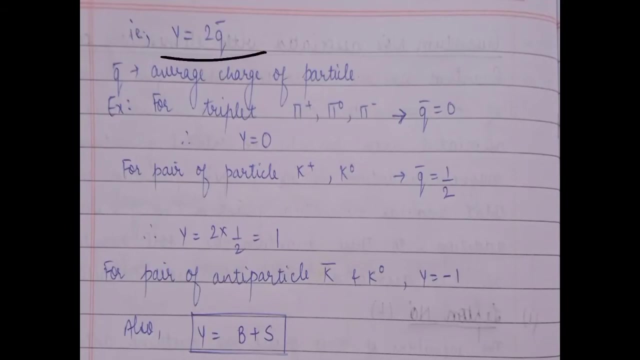 First we will, before that we will study the hypercharge. Hypercharge is also a quantum number whose value is twice the average charge of the numbers of the groups. that is, y is equal to 2q bar, where q bar is the average charge of the particle. For example, if we consider the triplets pions, pi plus, pi naught, pi negative- 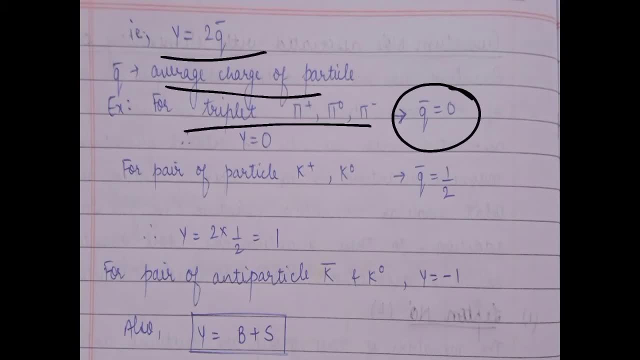 for them the average charge is equal to 0.. In this example we get: hypercharge is equal to 0 and for pair of particles, kions, k positive and k naught, we have average charge equal to 1. by 2, therefore, our hypercharge becomes equal to 1.. 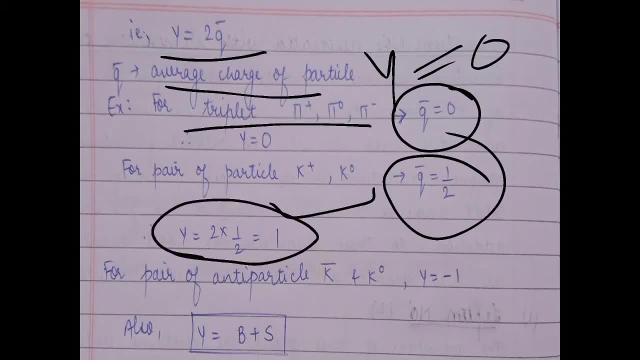 Similarly, for the pair of anti-particles of kions we have the hypercharge equal to minus one. We can also find out hypercharge by adding baryon number to that. We will see that in this example we will baryon number and strangeness quantum number. We will further study about the strangeness. 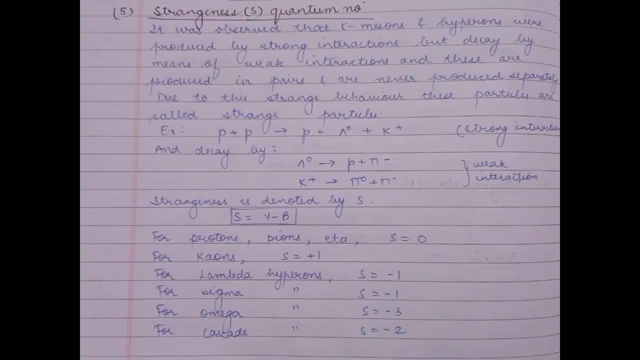 quantum number. Now it was observed that the k mesons and hyperons were produced by strong interactions. They were produced by strong interactions, but they decayed by means of weak interactions And due to this strange behavior they were called strange particles. 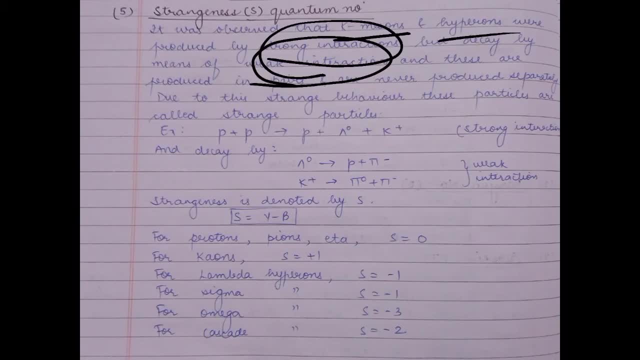 That is, for example, the lambda naught, was produced by the strong interaction, by this reaction, but it decayed by weak interaction through this equation. So they were called as strange particles because of this, This strange behavior, since they were produced by strong interaction but decayed by weak 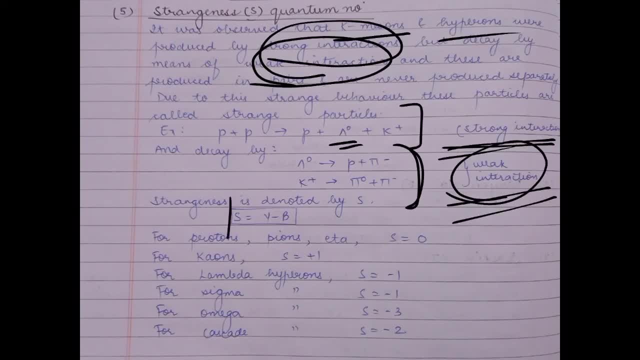 interaction. Now, strangeness, can be calculated by this formula, that is, y minus b, where y is the hypercharge and b is boron number. For protons, pions, eta s is equal to 0.. For kaons, s is equal. 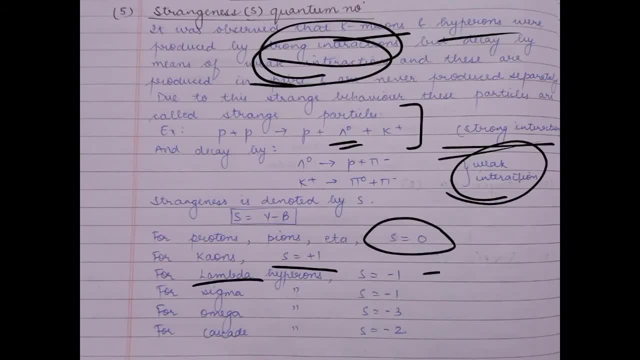 For lambda hyperons, it is equal to minus 1.. For sigma hyperon, s is equal to minus 1.. For omega hyperon, s is equal to minus 3.. And for cascade hyperon, it is equal to minus 2.. 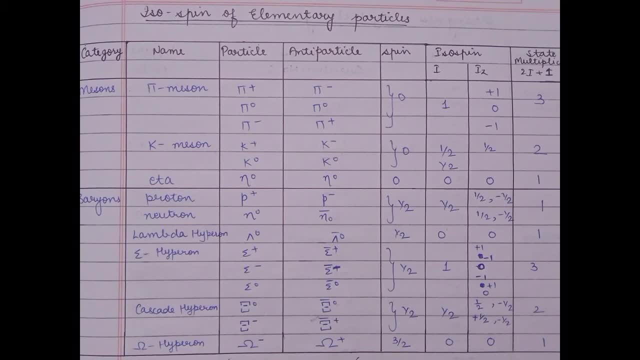 Now we will see isospin of elementary particles. First we will see the mesons. We will consider pi mesons which occur in triplet state. Now we know that Isospin of elementary particles, Isospin of elementary particles. 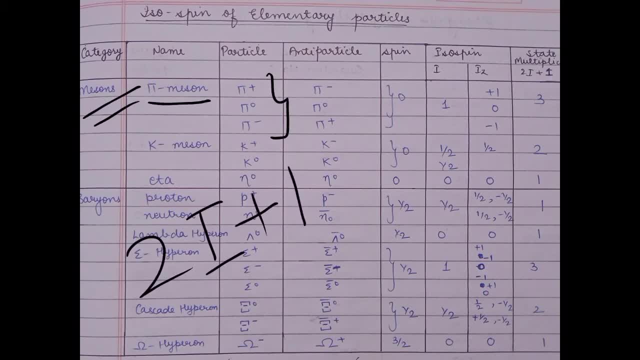 Isospin can be calculated by this formula: 2: I plus 1, which will be equal to number of triplet states, which is equal to 3 for pi mesons. Now here isospin will become 3 minus 1 divided by 2, which is equal to 2 divided by 2, equal. 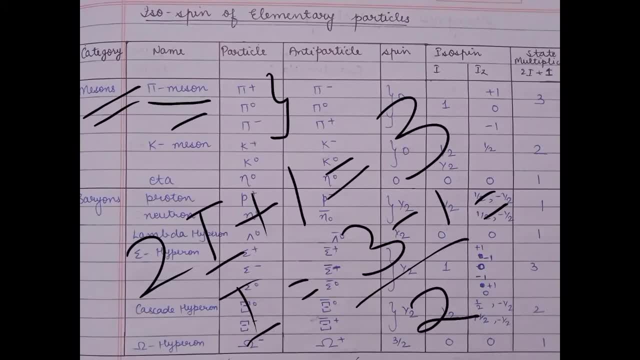 to 1.. So we get that isospin for pi mesons is equal to 1.. Similar to quelle room, Stirring motion, maturation and notation. Now we should see a critical 1.. Now, similarly, the k mesons occur in duplets, so their isospin is equal to 1 by 2 by the formula. 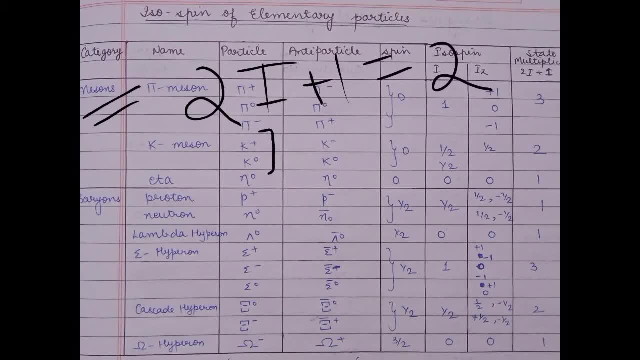 2i plus 1 equal to 2.. So similarly we can find out the isospin of all the elementary particles, and isospin is represented by i and its iz is the third component of isospin, whose value lies between minus i to plus i. Therefore, isospin for pions is plus 1 to minus 1 and the state 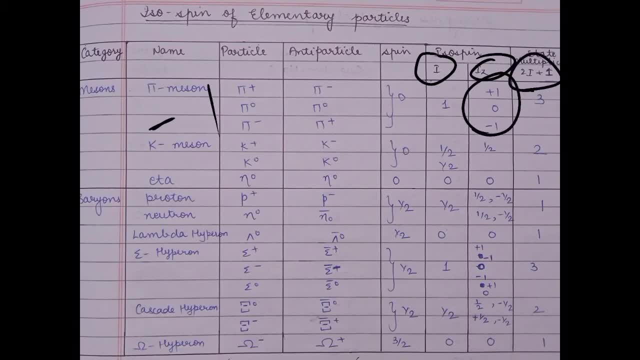 multiplicity can be found out 1 by 2i plus 1, formula which is equal to 3.. So we have 3 multiplets of pions. Similarly, where we have 2 multiplets of kaons, and therefore its isospin is 1 by 2 and the spin multiplicity. 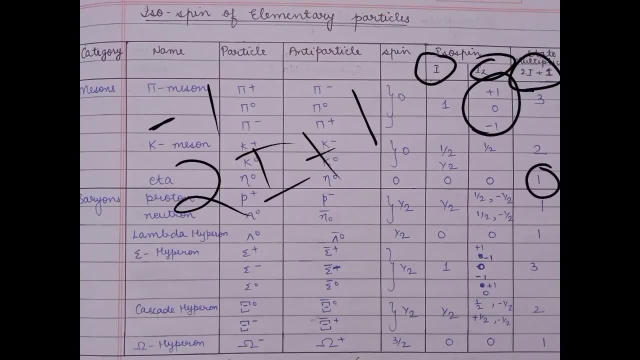 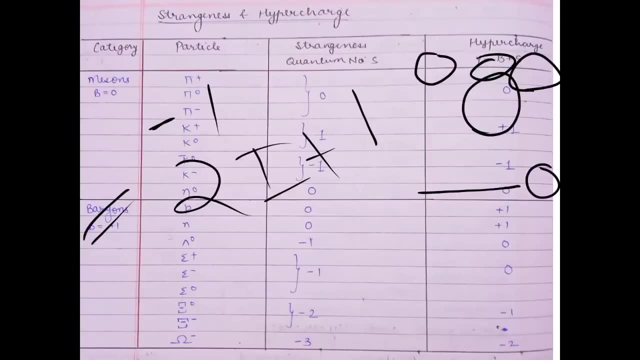 of eta is equal to 1.. Therefore its isospin is 0.. Similarly, we can find out the isospin number for all the baryons: 1 by 2i plus 1, formula which is equal to 3.. So we have 3 multiplets of pions. Similarly, 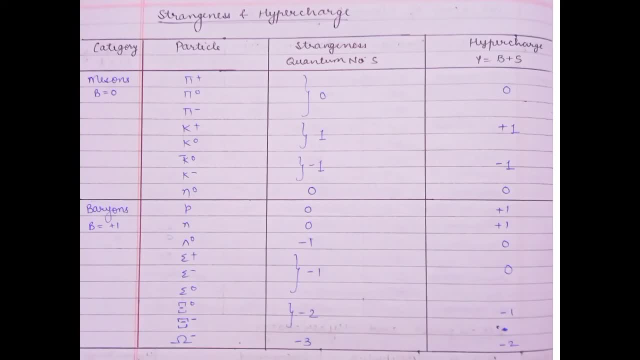 we can see the strangeness and hypercharge for the mesons and baryons, For pions, all the pions strangeness number is equal to 0. Therefore their hypercharge is also equal to 0, because hypercharge is equal to baryon number plus strangeness, quantum number, Since mesons are. 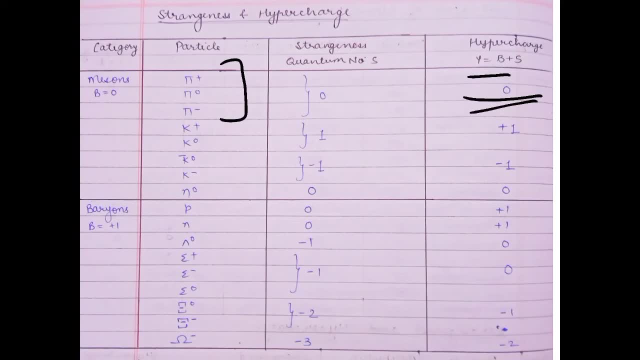 not the baryons. therefore, baryon number is equal to 0 and since the strangeness is also equal to 0, therefore their hypercharge becomes equal to 0.. For kaon particles, the strangeness is equal to 1 and for kaon antiparticles the strangeness is equal to minus 1.. Therefore, 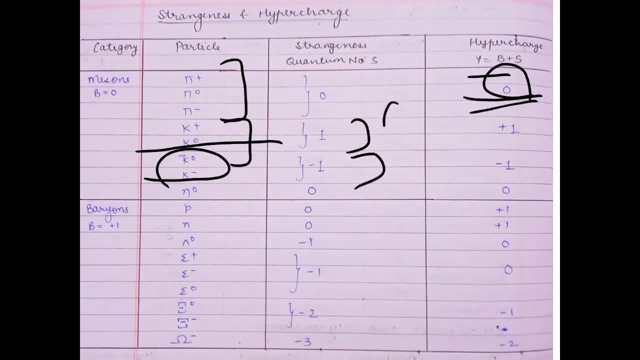 their hypercharge becomes 0 plus 1, equal to plus 1, and for antiparticles hypercharge is equal to 0 minus 1, equal to minus 1. here 0 becomes because these are not baryons. baryon number is only for baryons and since these are mesons, therefore for them b is equal to 0. now for eta. 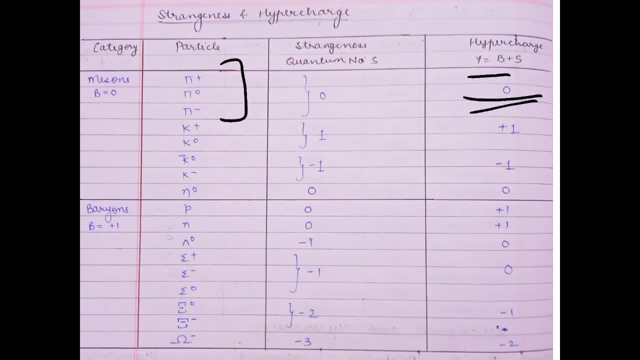 the strangeness is equal to 0 and its baryon number is is also equal to 0, therefore its hypercharge becomes 0. now for baryons, for protons and neutrons, that is nucleons, the strangeness is equal to 0 and since they are baryons, therefore their baryon number is plus 1. 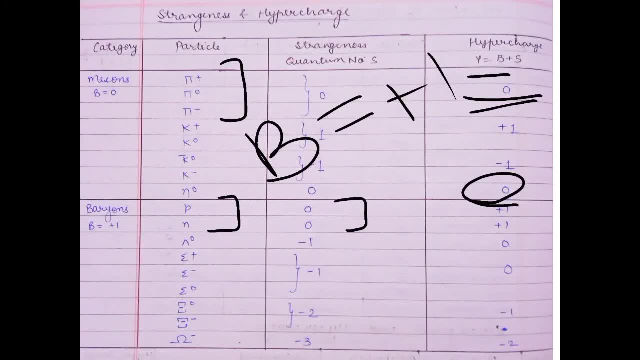 therefore, their hypercharge becomes plus 1 and the baryon number and the strangeness quantum number for lambda hyperion and for sigma Hyperion is equal to minus 1 and since these are baryons, therefore their baryon number is equal to plus 1. therefore, the hypercharge becomes plus 1 minus 1, equal to 0. therefore, 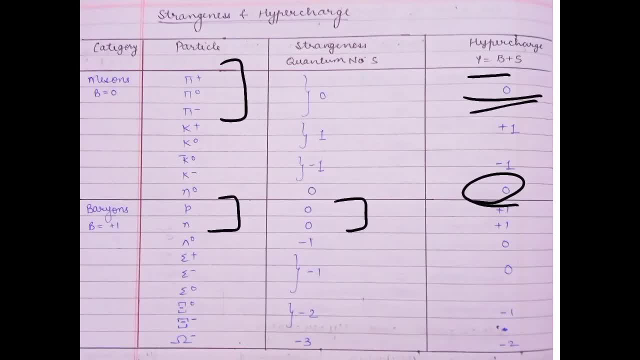 the hyper charge for sigma and lambda baryons. lambda hyperons becomes equal to 0. now for cascade strangeness. quantum number is equal to minus 2 and since they are baryons, therefore, the hypercharge becomes plus 1 minus 2, which is equal. 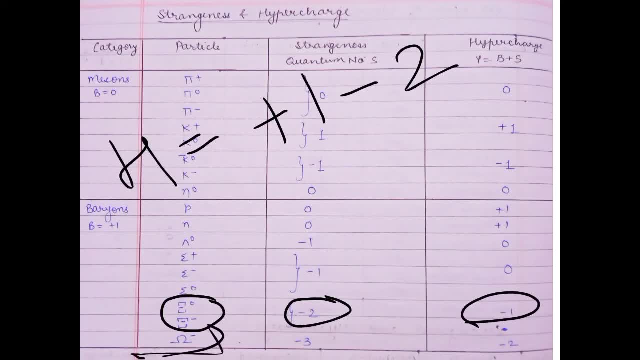 to minus 1, and for omega hyperion. and for omega hyperion, strangeness quantum number is minus 3. therefore its hypercharge becomes plus 1. for baryon number minus 3. for strangeness quantum number, therefore, the hypercharge becomes minus 2. so in this video we studied about the quantum. 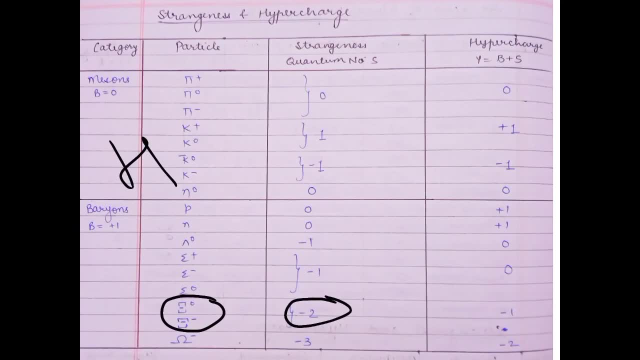 number. i hope it is clear for you. so we will end up here. i hope you like the video. if you like the video, please subscribe it and share the video. thank you.